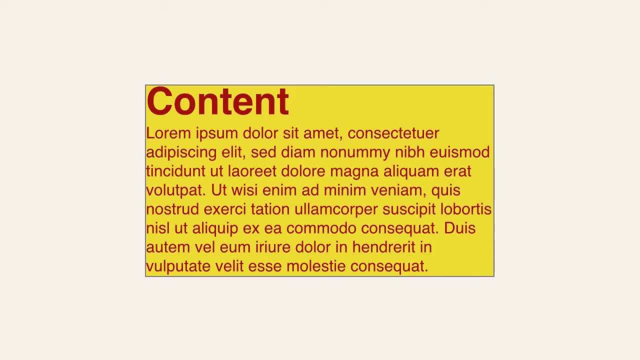 width for this content box. The height of the element, unless specified, is going to be determined by the amount of content that we have inside this box. So if our paragraph is longer, then our box is going to be taller. So, again at the base level, our width and height are determined by the content. 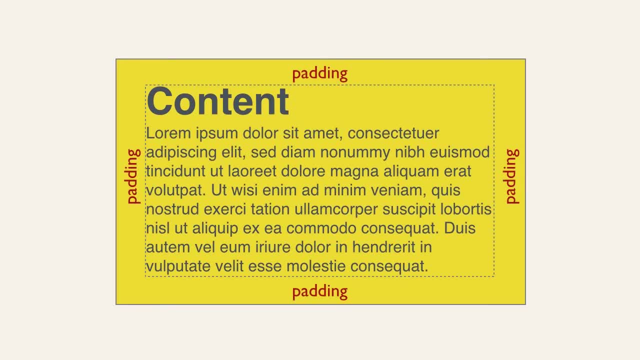 itself. However, once we start adding padding to our content, for example, as you can see here, our box is going to get larger. So if you set your box to a width of 100 pixels, for example, and then you add padding of 20 pixels, then the full width of your box is going. 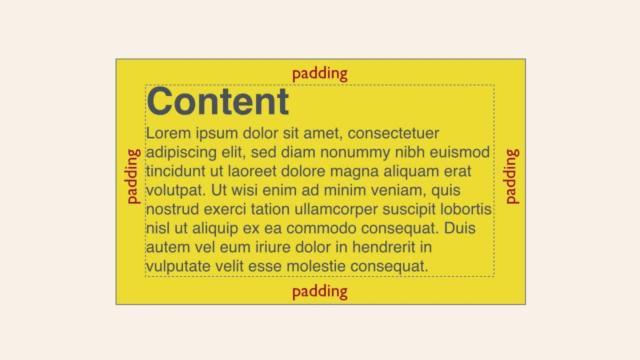 to be 140 pixels, because you'll have 20 pixels of padding on the left and 20 pixels of padding on the right. Now you might have thought that this happens the other way around. You might have thought that if we were to add padding to a box of content, that the content inside it would get. 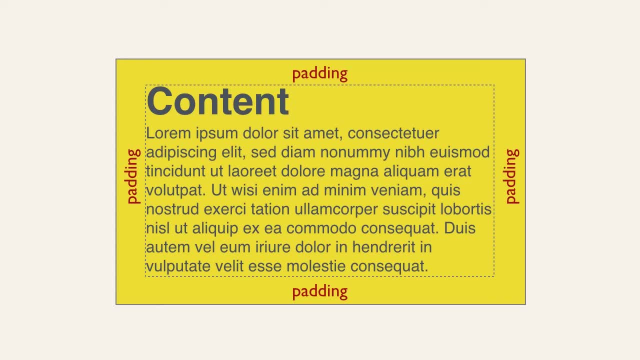 smaller and that's not the case By default. the content inside this box is going to keep the same width no matter what. But when we add padding and borders and margins, that width is going to get larger. So if we go back, when we see the content by itself, our box has a certain width. 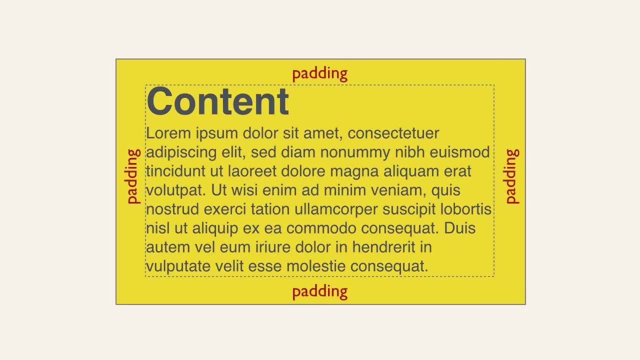 and height. But when we add padding, the width gets wider and the height gets taller by whatever amount we've placed for the padding property of this box. So if all four sides have a padding of 20 pixels, then our box is going to be 40 pixels wider and 40 pixels taller than it. 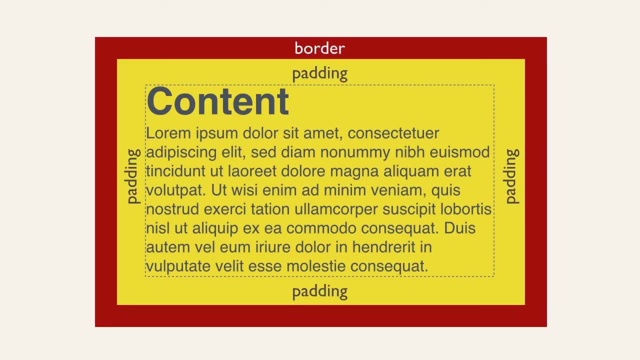 started out. Now, let's say we complicate this by adding a border. Let's say our border is maybe two pixels thick. Well, that's going to add four more pixels of width because we have the left border and the right border, both of which are two pixels thick, and it will also add four pixels of 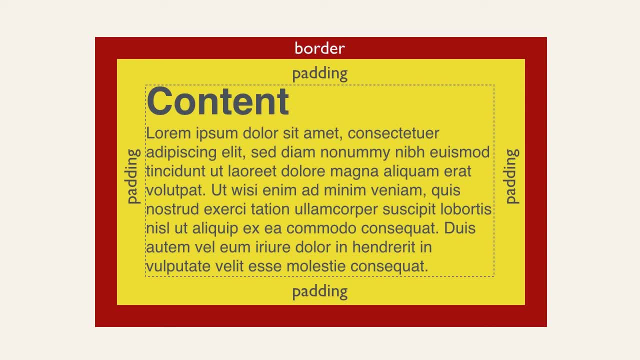 height. So, in addition to our content, we have 20 pixels of padding on the top, right, bottom and left, As well as a couple of pixels of border on the top, right, bottom and left. Then, if we don't, 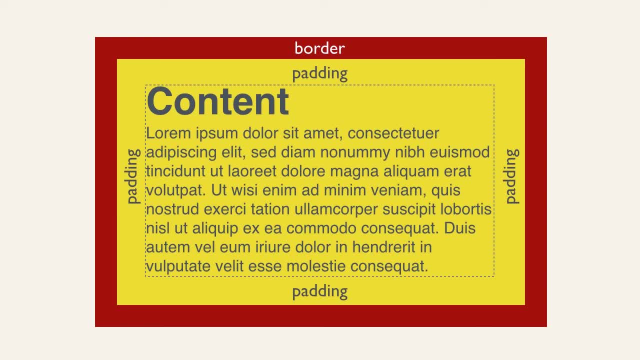 want this box bumping up against other boxes. if we want to put a little space around this box, that's going to extend the reach of this box even further. Now that we have this box pushing things to the side, this box is going to be taking up even more space in our browser. So if you're